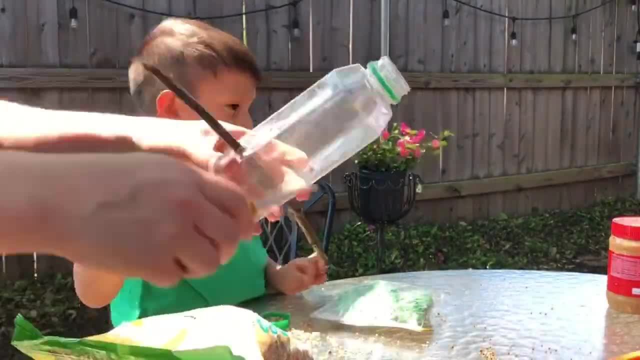 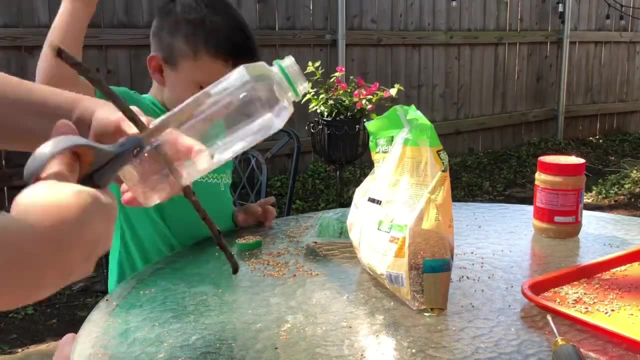 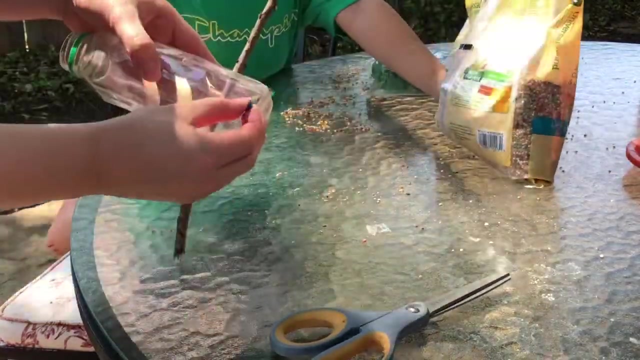 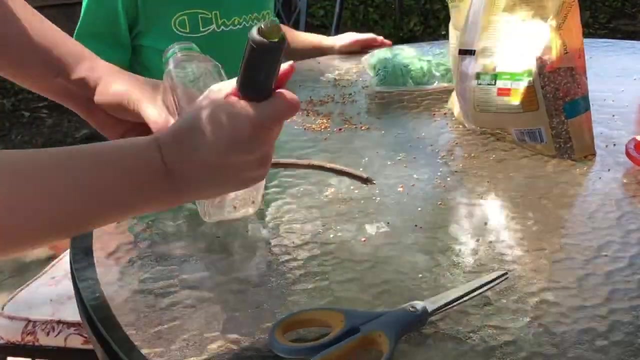 opening. I use the screwdriver to widen the hole big enough to fit scissors comfortably. The hole should measure about an inch in diameter. Now repeat these same steps on the other side. Keep in mind that you want to create a perch hole about an inch or an inch and a half above or below the first initial. 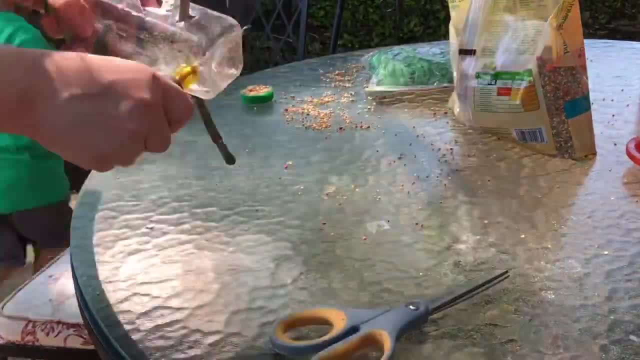 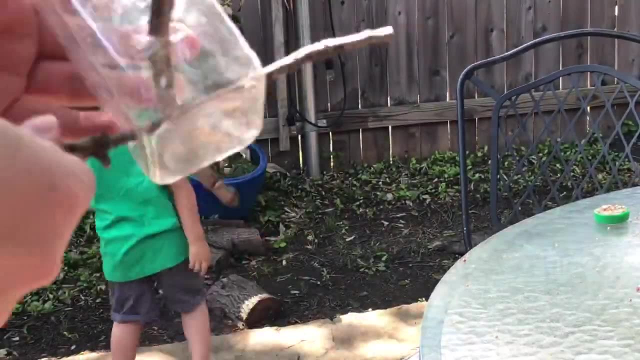 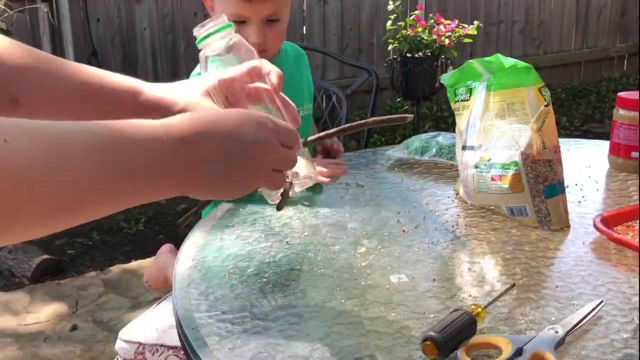 perch holes so that the sticks can fit all the way through. Once both sticks are through the plastic bottle, it should create a cross-like shape if you were to look at it from the bottom. And don't forget to create the feeding holes for the second perch sticks. 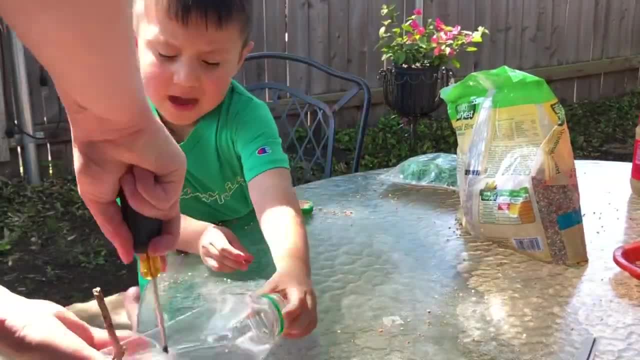 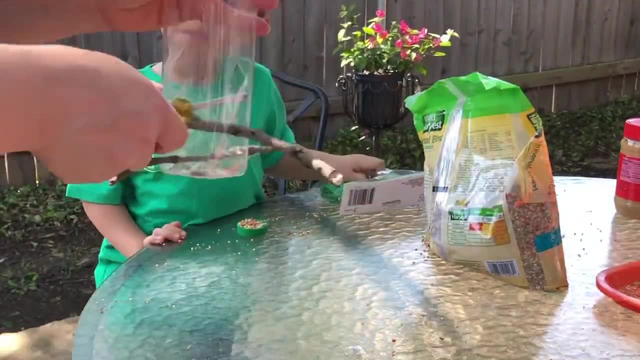 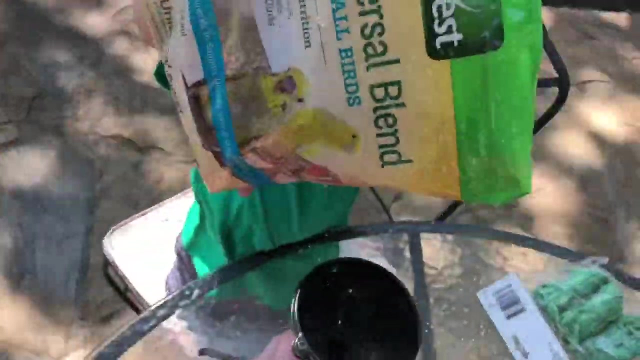 We're almost done- I promise We're done- with the first DIY bird feeder. The second one is a lot simpler. Now you're going to add your favorite bird seed and attach a string or a yarn at the opening of the plastic bottle. Screw the top on and that yarn or string is secured, and 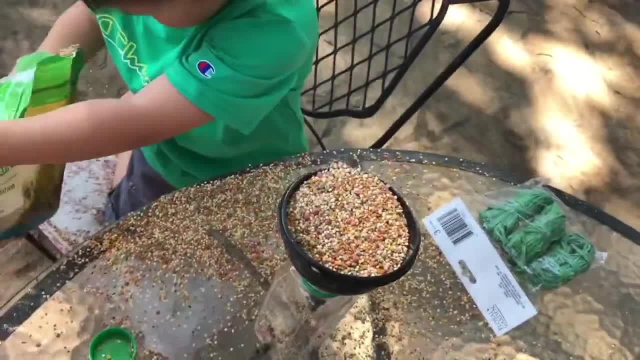 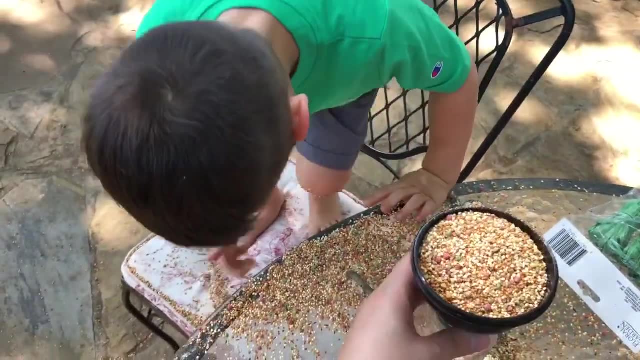 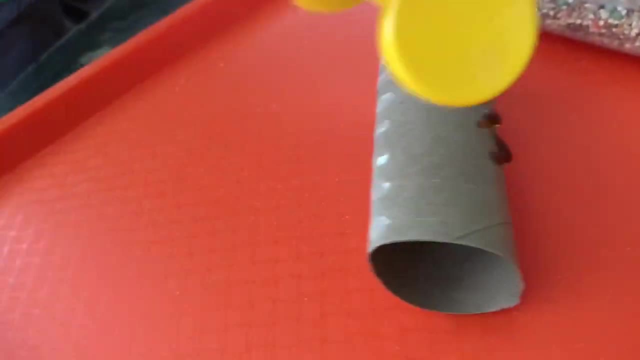 you can hang it from your favorite tree. And, as you can see here, we used just a little bit too much bird seed, but it was part of the fun and part of the built-in memories. On to the second DIY bird feeder. This one's a lot simpler and David, my toddler, was able to basically do most of the work. 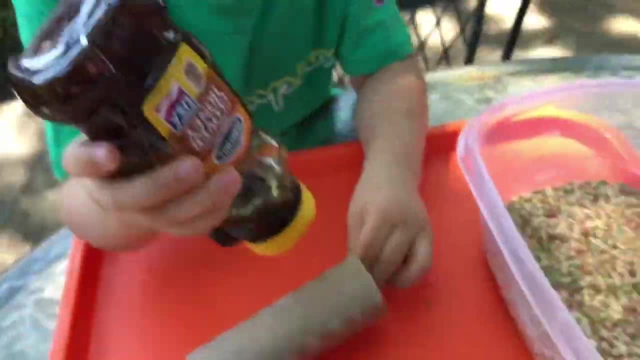 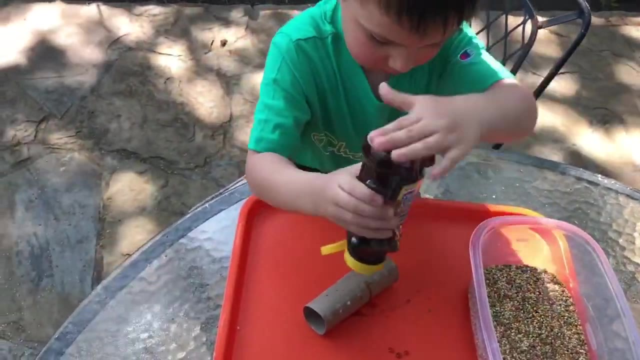 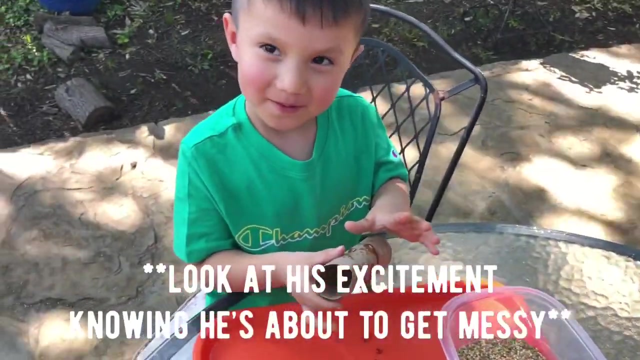 Here you're going to use an empty toilet paper roll, or even a paper towel, and just cover it first with honey or peanut butter and just make sure that it's completely saturated, so that the bird seed sticks pretty easily. Hey Mommy, What are you going to do? 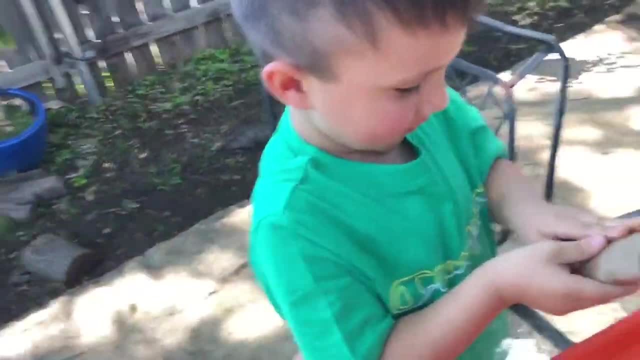 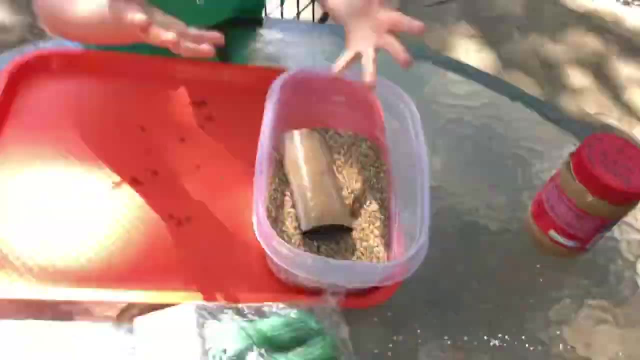 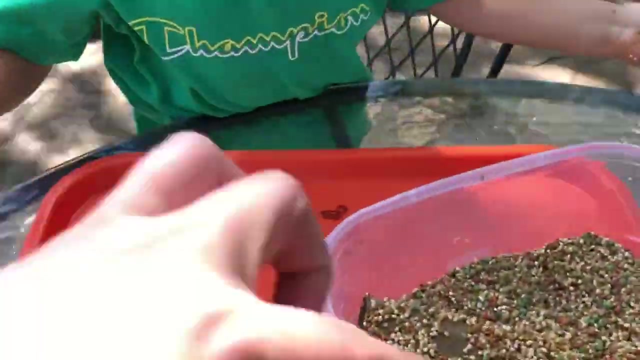 I'm going to do this And, as you can tell here, he is pretty excited about getting messy, and you know, just let him go for it. This is the bird seed that fell earlier and we just kind of put it in a little Tupperware. 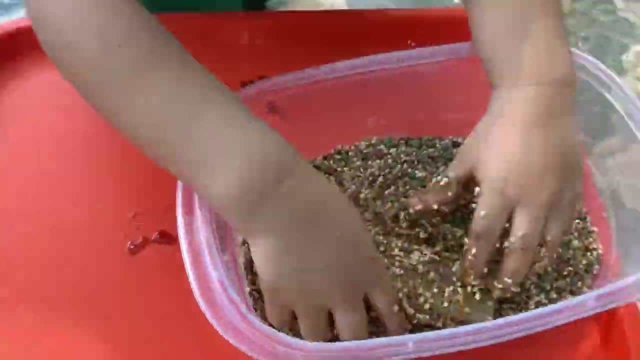 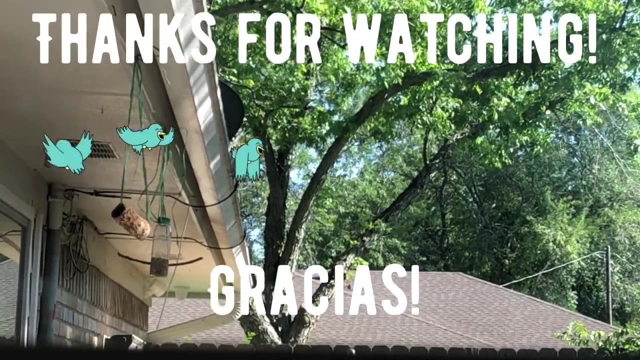 dish, rolled it around and we were able to string some yarn through it, and that was it. We hung it and called it a day. We didn't have to worry about it, We just had a good time and it was a great day. And it's been a fun day. Thank you, Thank you, Thank you. . . . . .